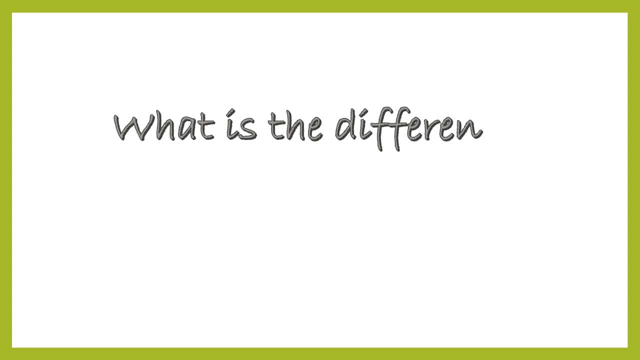 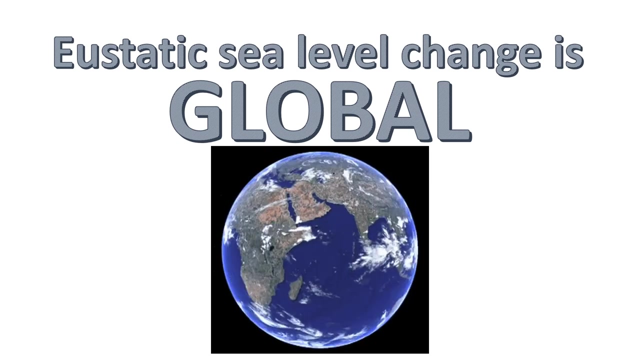 What's the difference between isostatic and eustatic sea level change? Eustatic sea level change is global sea level change. This means that everywhere in the world is equally affected by it and sea levels rise by the same amount in all coastal areas. 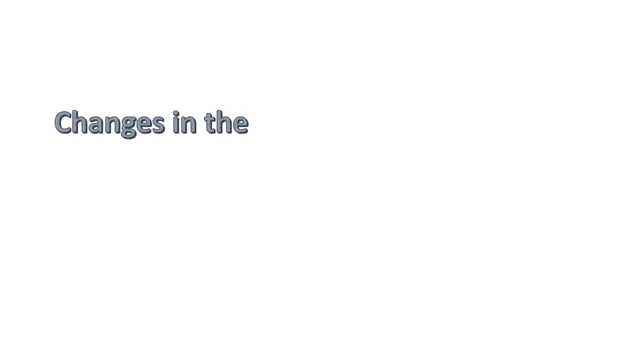 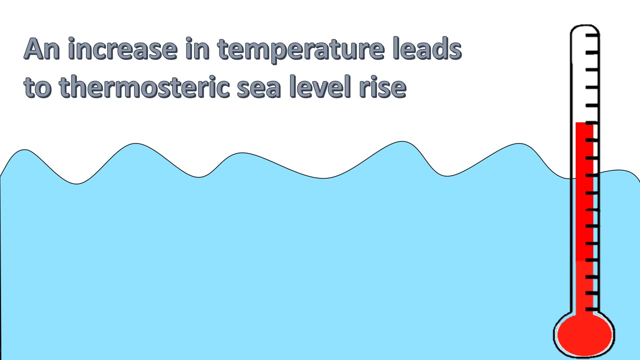 One cause of eustatic sea level change is changes in the volume of water actually in the sea. An example of what causes this is climate change. Increased temperatures lead to thermoesteric sea level rise, which is also known as thermal expansion. This is when water molecules are heated and move further apart from each other, So the volume of water expands and the sea level rises. 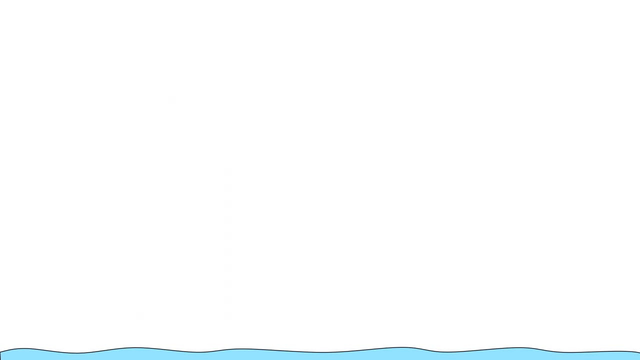 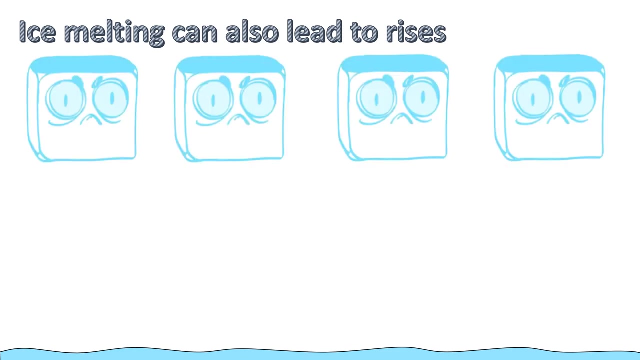 Higher global temperatures due to climate change also causes glaciers and ice sheets to melt. Water that was locked up in ice melts and the melt water enters river systems. It will eventually melt. It will reach the mouth of the river and be stored as liquid water in the sea. 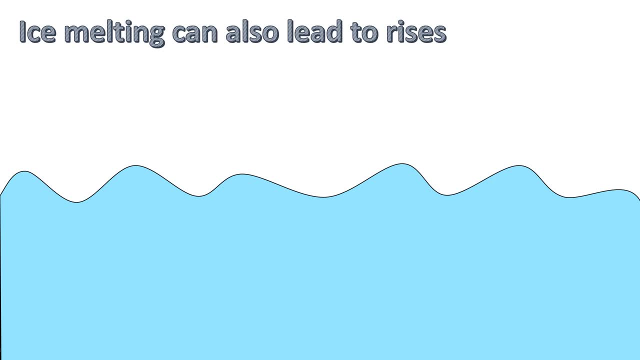 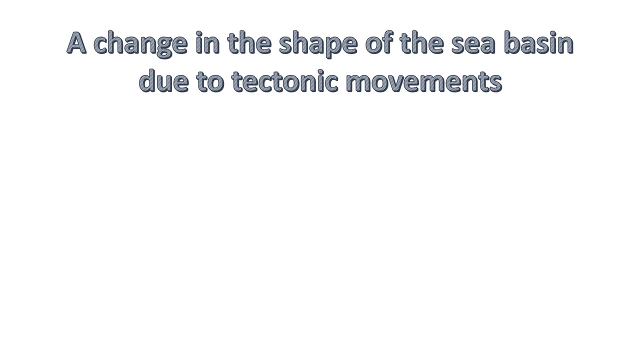 The volume of water in the sea increases. therefore, sea levels rise. The opposite can happen in an ice age Eustatic. sea level change can also be caused by changes in the shape of the sea basin due to tectonic movements of the Earth's crust. 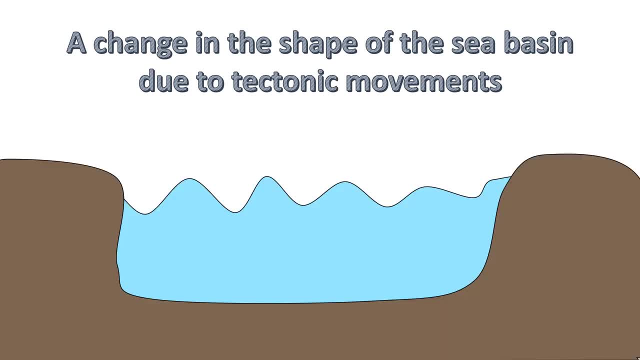 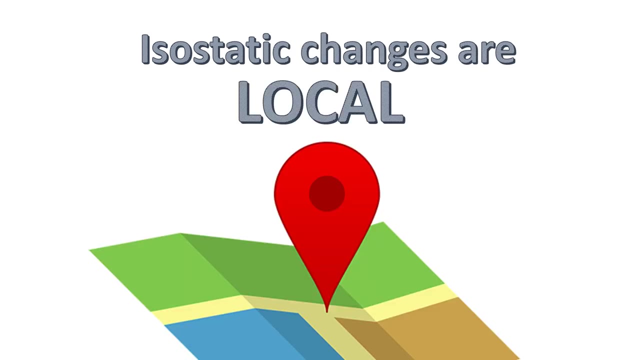 This then changes the volume of water able to be held in the ocean. For example, sea floor spreading increases the size of the sea basin, Leading to a greater volume. therefore, sea level falls. Isostatic changes are local changes. This means that the sea level change only affects one area. 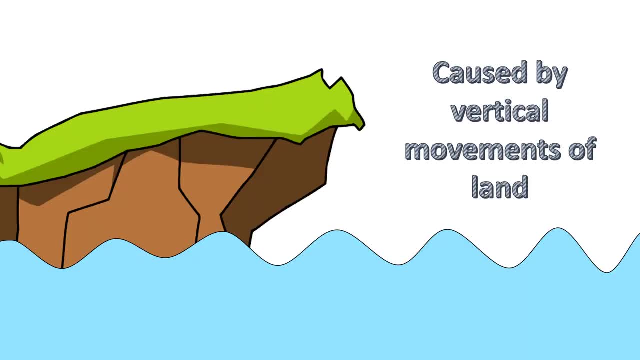 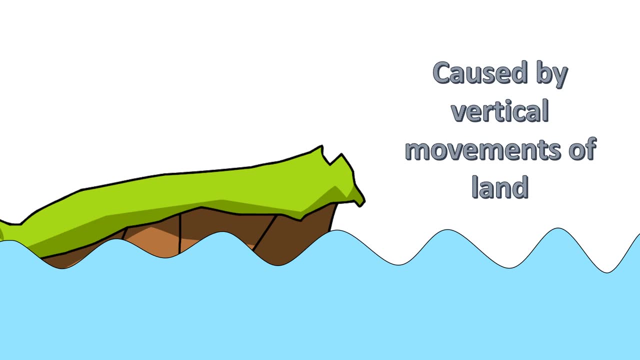 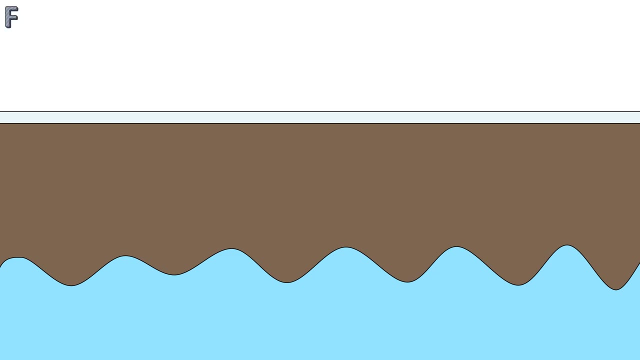 Isostatic change is caused by vertical movements of land. Movement upwards causes sea levels to fall, whereas downwards movement of land causes sea levels to rise. One cause of land movement is compression or decompression. This can be caused by glaciers. When glaciers form, their weight pushes down on the land, causing it to move down. 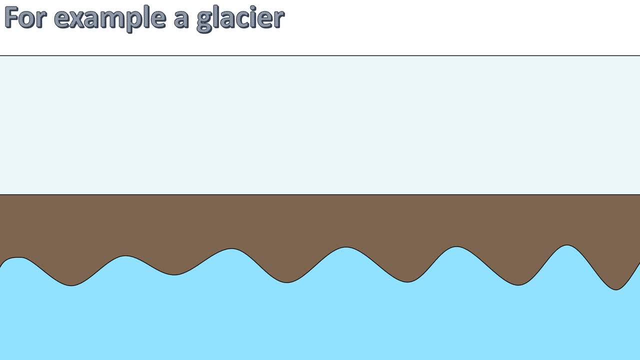 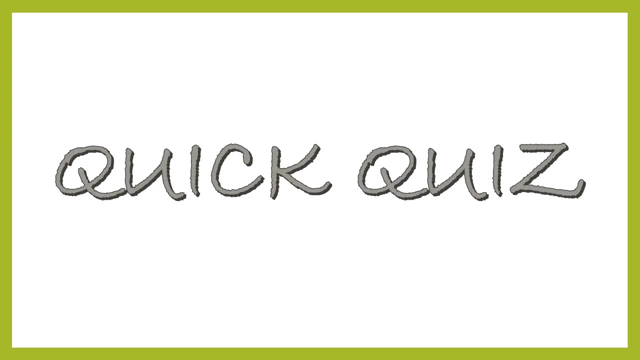 However, when the ice melts, the land no longer has that pressure pushing down on it, so the land rebounds and rises. So now we have a quick quiz and it's time to test your knowledge. Six statements will appear and you need to match them to either isostatic or eustatic sea level change.